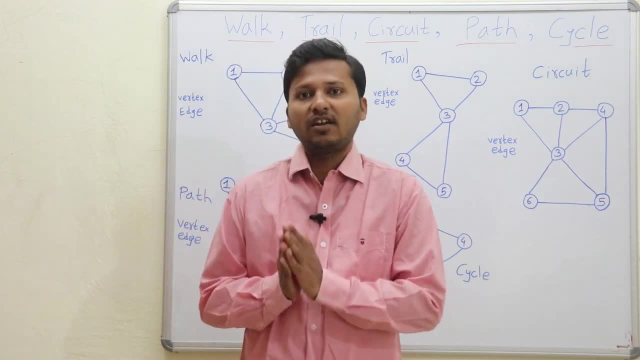 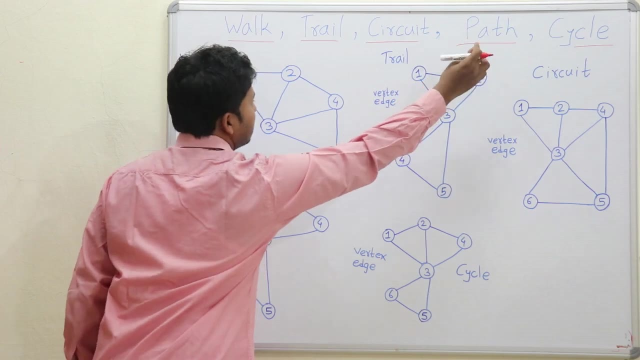 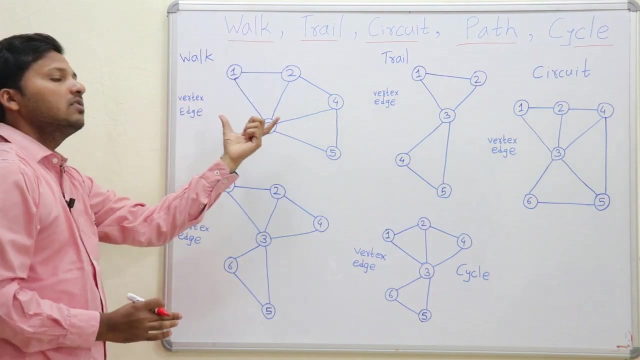 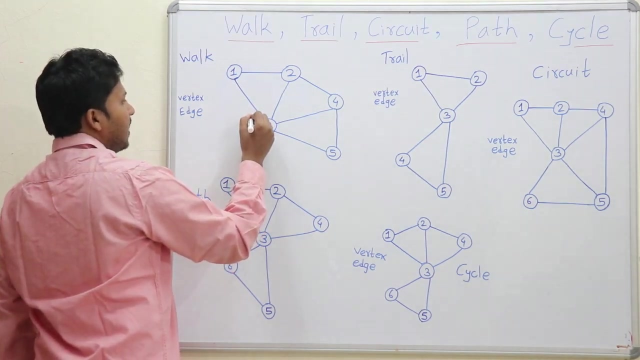 Hello friends, today we are going to see some terms in graph theory. So those terms are walk, trail, circuit, path and cycle in a graph. So let's first see what is a walk in a graph. So when you traverse a graph, you can traverse it in any way, like here, starting from vertex 3. 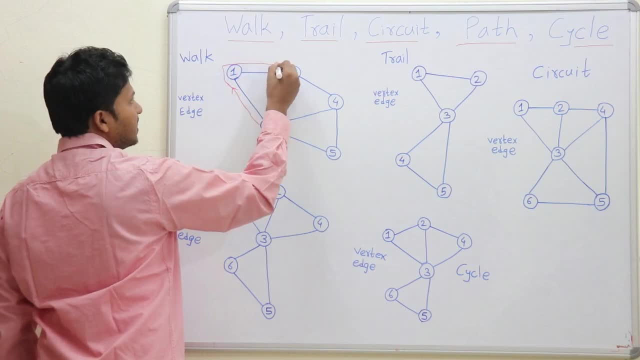 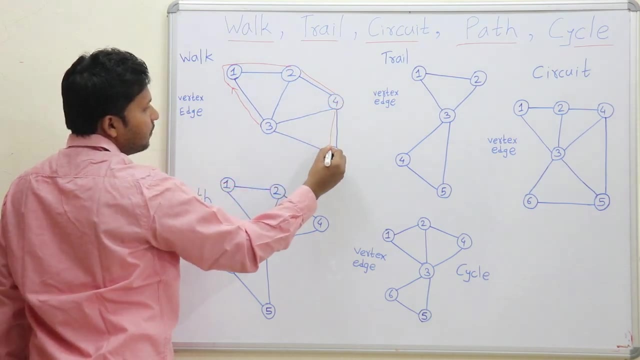 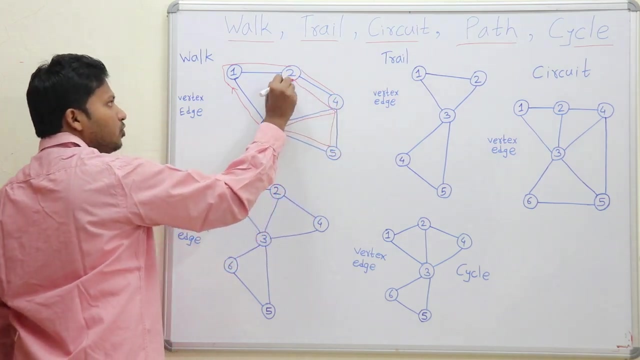 to vertex 1, then from vertex 1 to 2, then from vertex 2 to vertex 4, then from vertex 4 to 5,, 5 to 3, then again from 3 to 4, again from 4 to 2, again from 2 to 1.. So in this way you can. 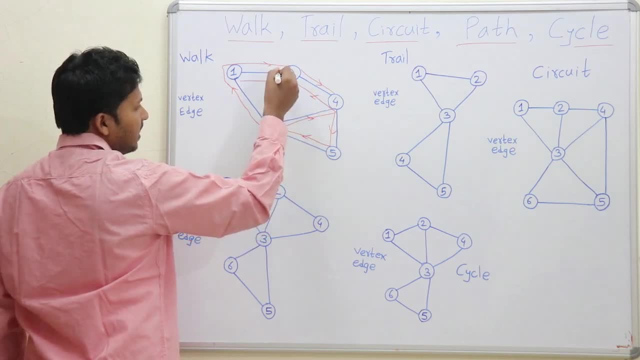 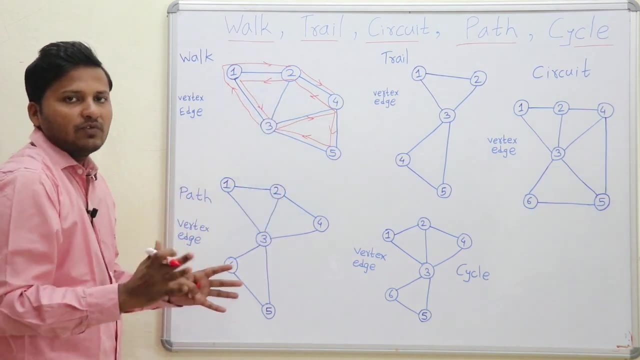 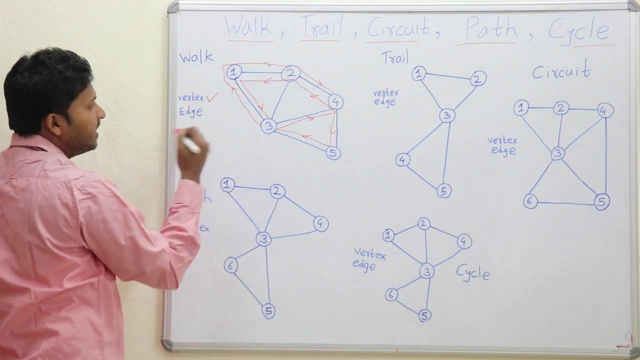 traverse the graph as you wish. So this is the path again from 1 to 3.. So for a walk, you can traverse the graph as you want, Means the vertex in the traversal can be repeated and the edges can also be repeated. So see, the vertex and edges can be repeated when you are. 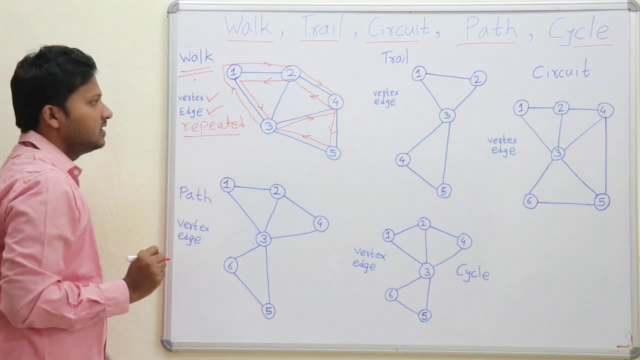 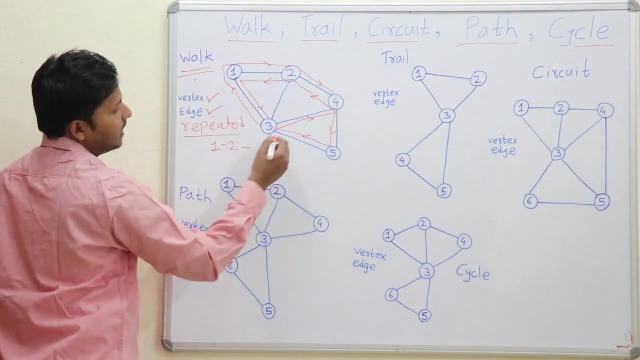 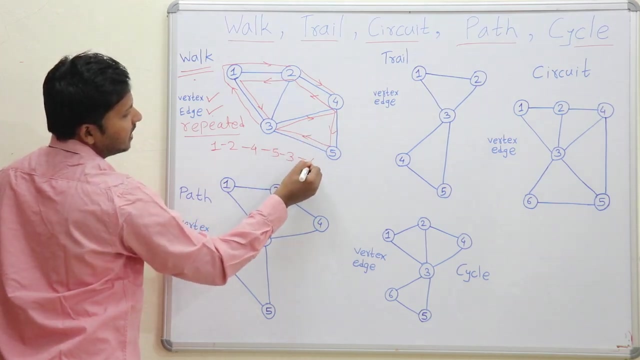 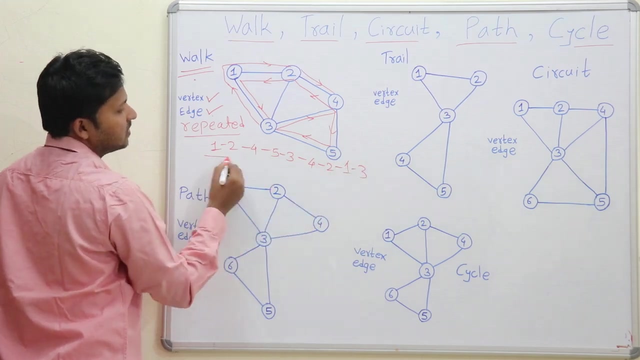 performing a walk, So this is called as the walk. So I will write the walk here, See 1, then 2, then we went to 4,, 5, 3,, 4, again 2, again then 1 and 3.. So this was our walk in this graph. 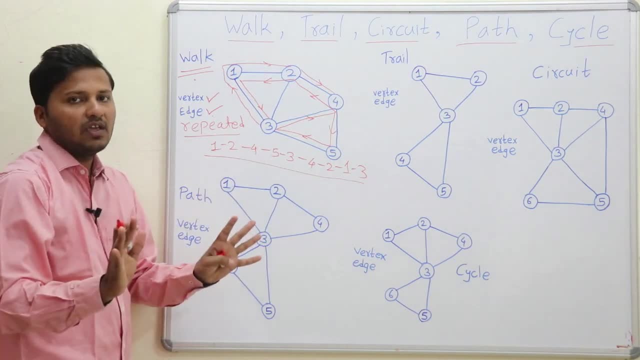 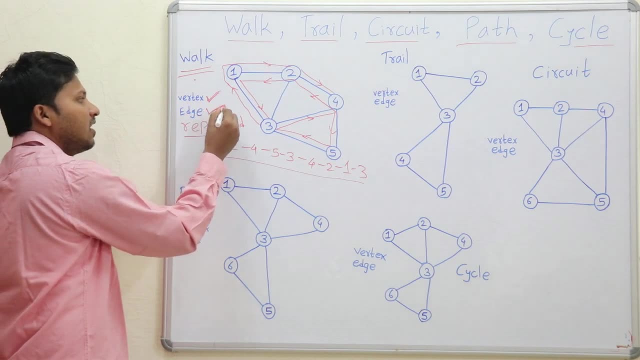 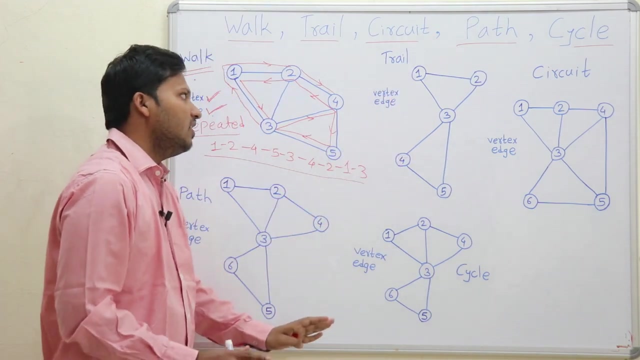 So in a walk you can traverse in any way, whatever you wish. The vertex are allowed if it is repeated, and the edges are also allowed. Now let us go to trail. So in a trail there is one condition. That condition is: vertex can be. 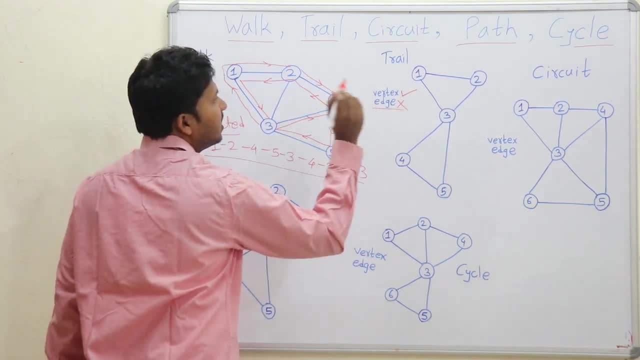 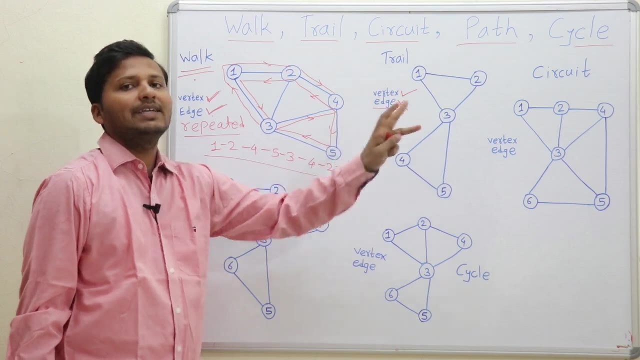 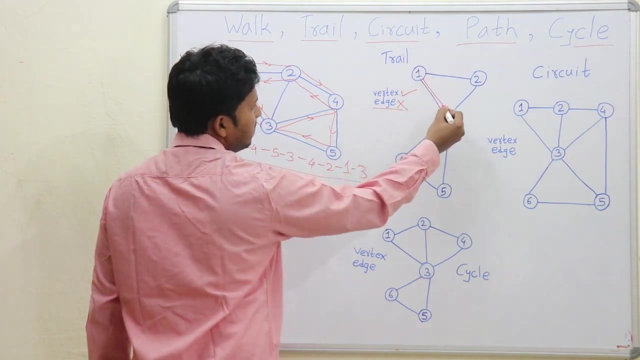 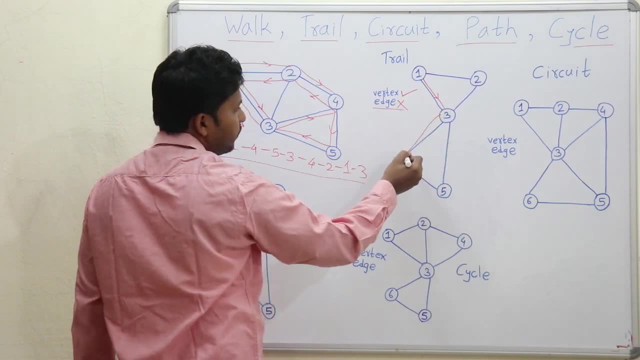 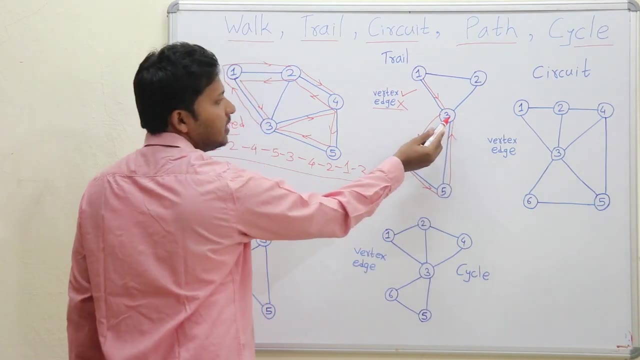 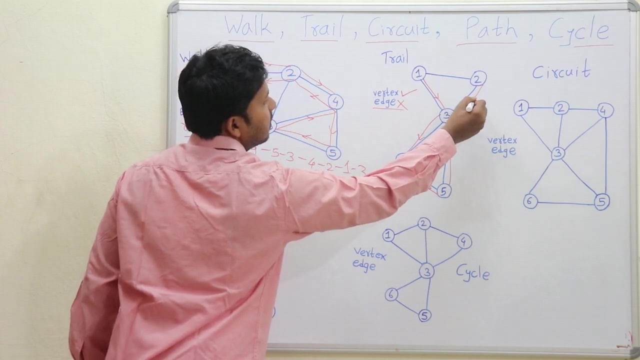 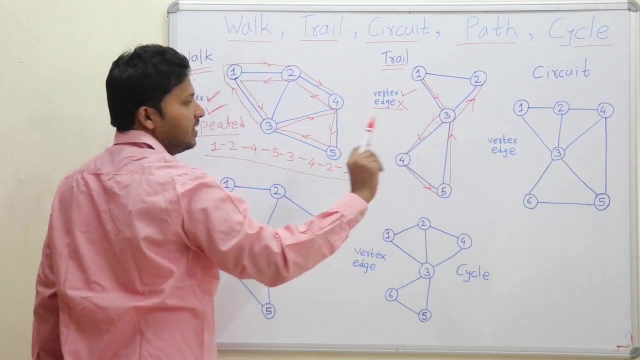 then from 1 to 3, then from 1 to 3, then from 3 to 4, then from 4 to 5, 5 to 3 again. See now the vertex 3 is repeated, Now from 3 to 2.. Okay, So this is a trail. here Means the vertex can be repeated. 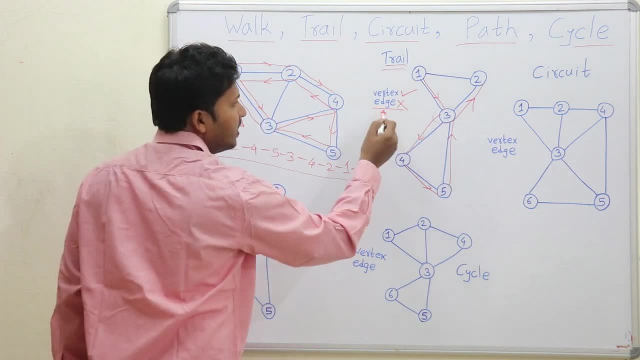 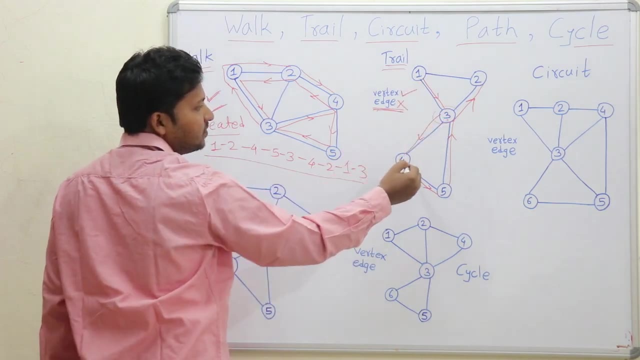 It is allowed. Any number of vertices can be repeated, but the edges should not be repeated. Okay, Means suppose from 1 to 3, and again we went from 3 to 4.. So we cannot go back from 4 to 3. 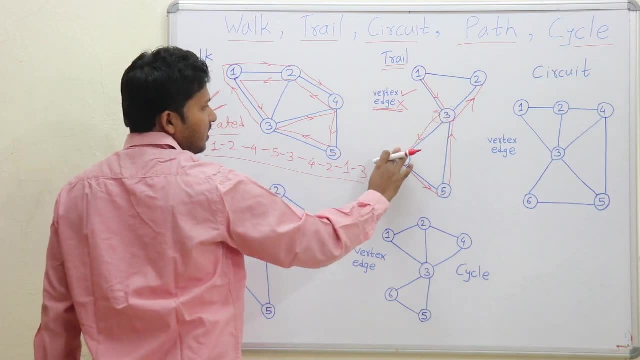 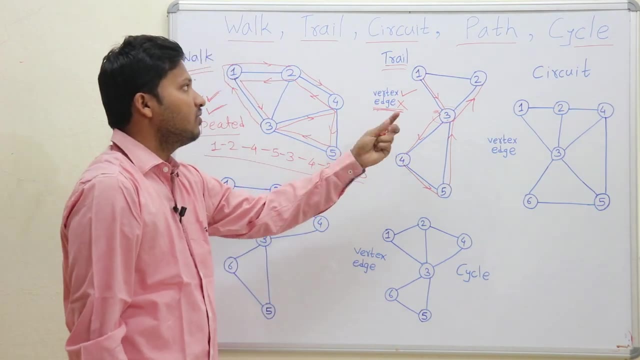 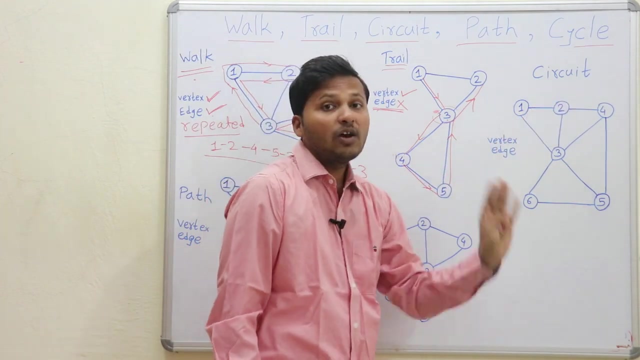 because this edge is repeated Right, So the vertices can be repeated, but the edges should not be repeated in the traversal, And that traversal is called trail. Now let us go for circuit Now. a circuit satisfies every condition of a trail, So let us go to trail Now let us go. 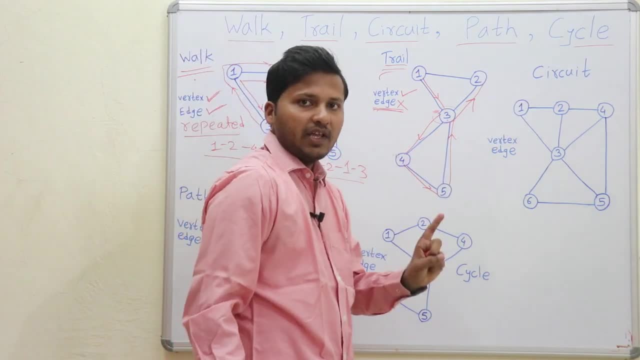 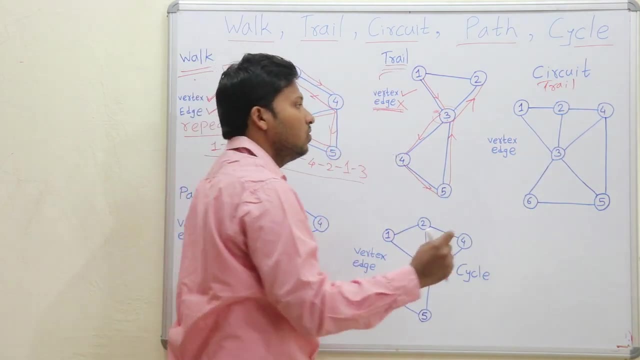 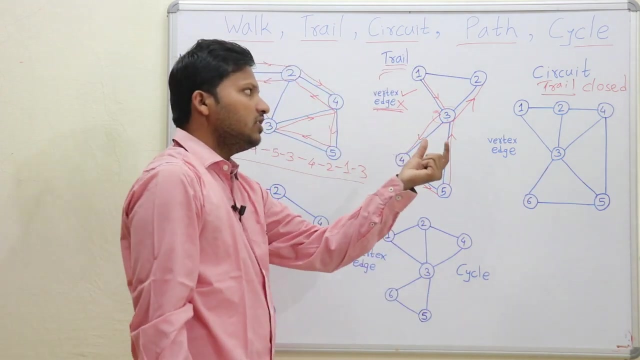 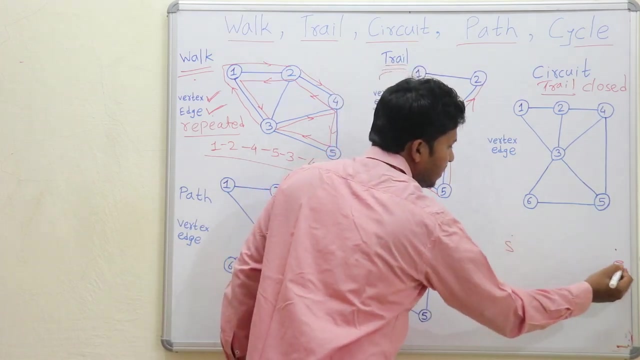 to the condition of a trail Means a circuit is a trail, with an extra condition. So that condition is: this trail should be closed. Okay, So this trail should be closed Means the starting vertex and the ending vertex should be the same. Okay, The starting vertex and the ending vertex should. 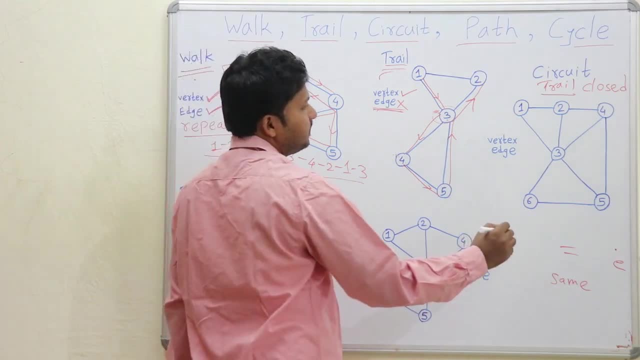 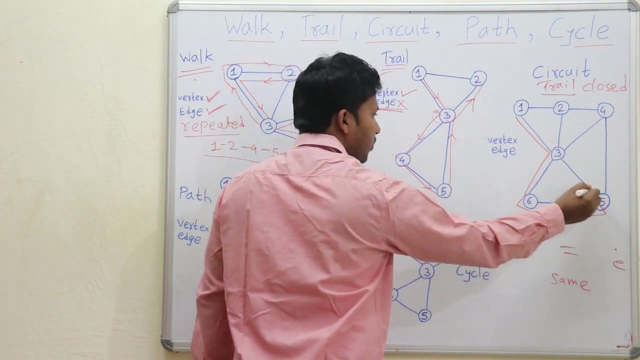 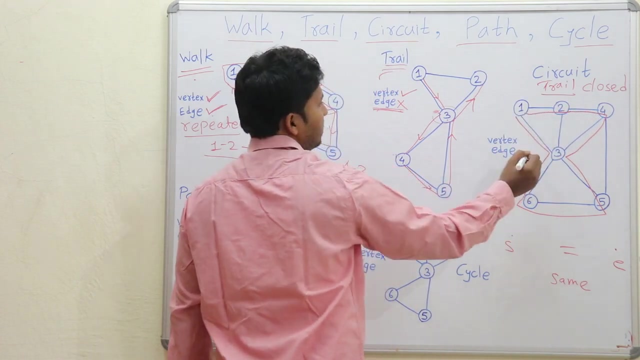 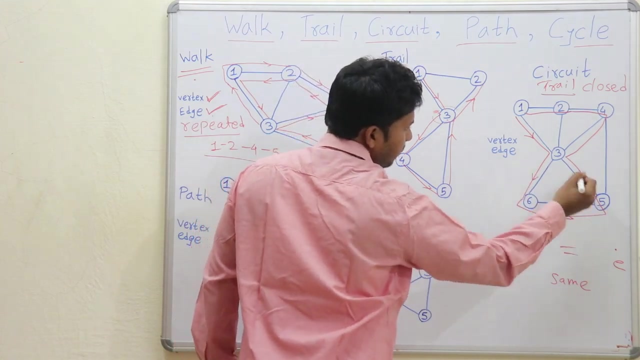 be same in the traversal. So let us see. So: start from 1.. So going from 1 to 3,, 3 to 6,, 6 to 5.. Again, from 5 to 3.. Then go from 3 to 4, 4 to 2 and 2 to 1.. So the circuit is see: 1 to 3 to 6 to 5,, 5 to 3,. 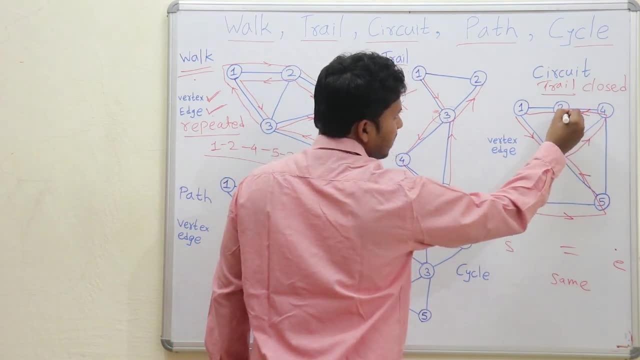 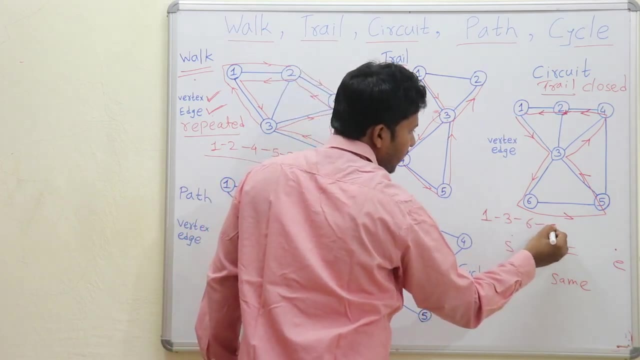 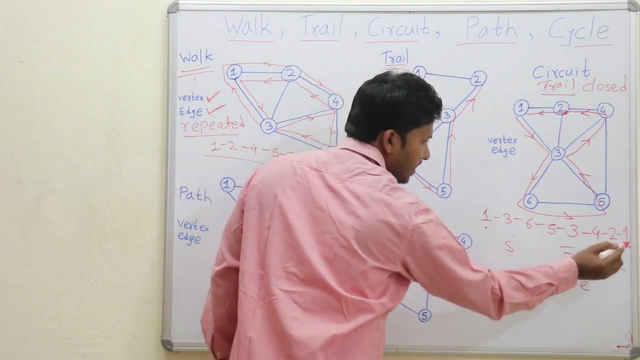 3 to 4,, 4 to 2 here And 2 to 1.. So let us write: see 1,, 3,, 6,, 5.. Again, 3,, 4,, 2 and 1.. So the starting and the ending. 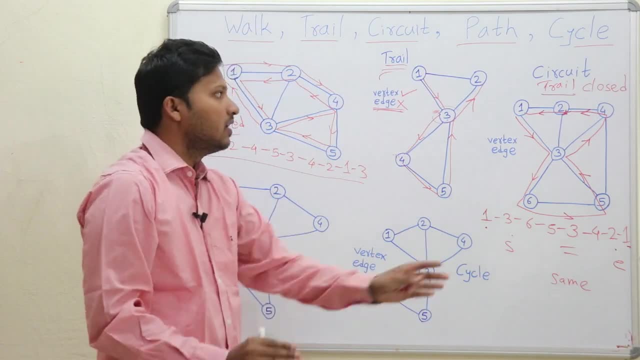 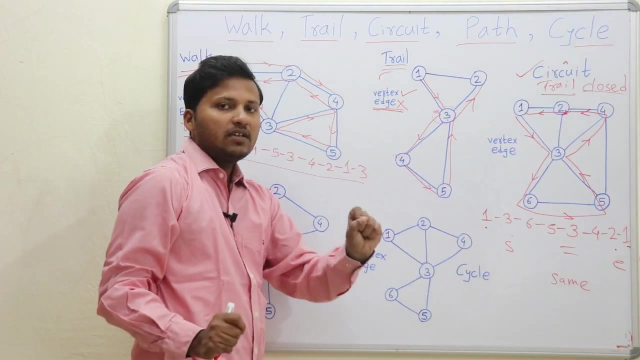 vertex is same Means the trail is closed And when the trail is closed it is called as the circuit. So a circuit is a trail. which is closed Means a circuit satisfies all properties of a trail, So the trail is closed And when the trail is closed it is called as the 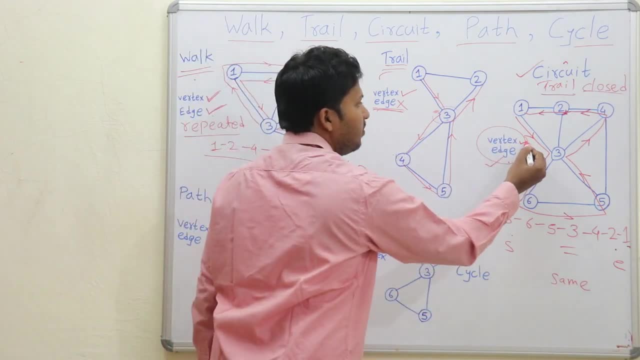 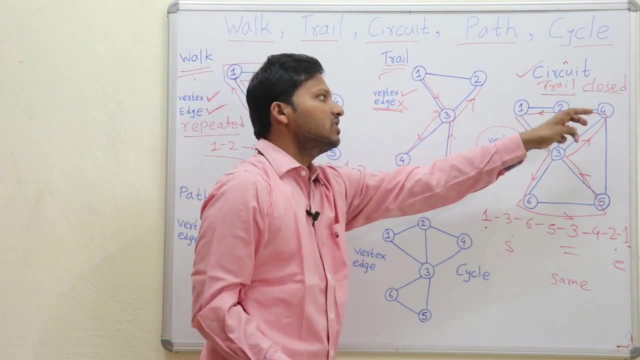 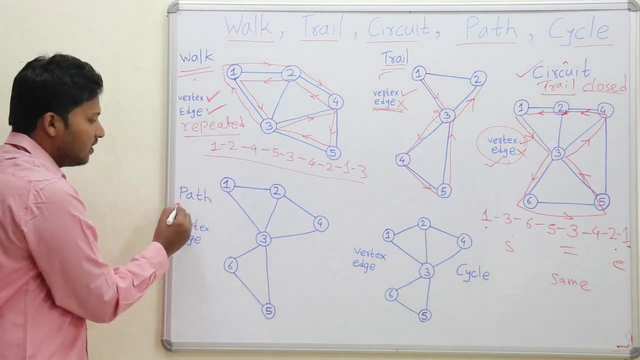 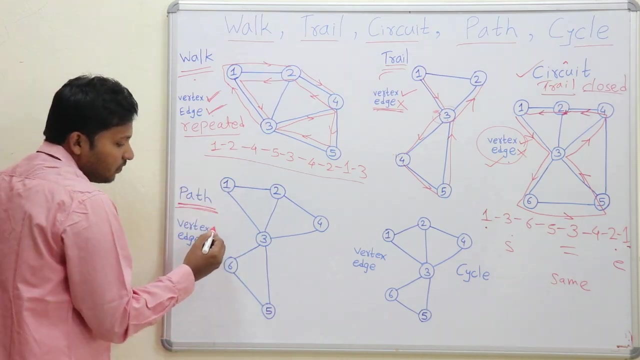 properties of the trail Means vertex can be repeated, but the edges cannot be repeated in the circuit. But that traversal should be closed. Okay, So this is called as the circuit. Now let us go to a path in a graph. So for the path there are conditions like vertex cannot be repeated and 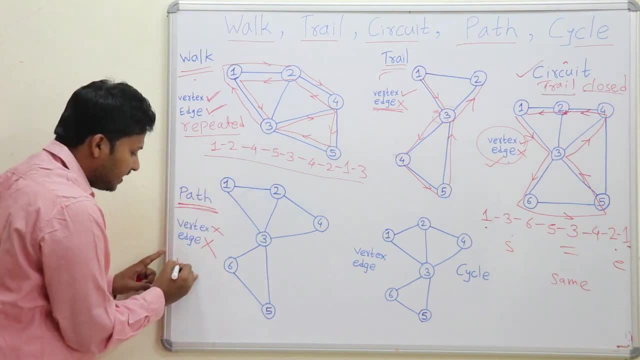 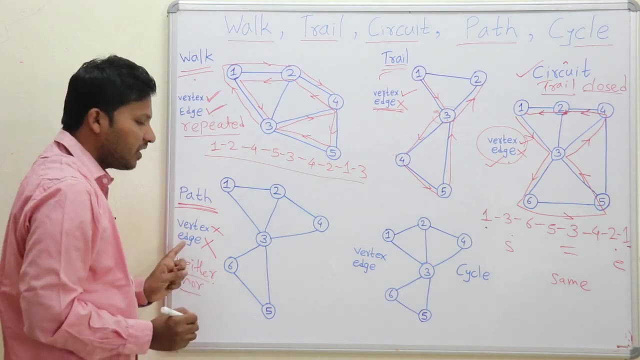 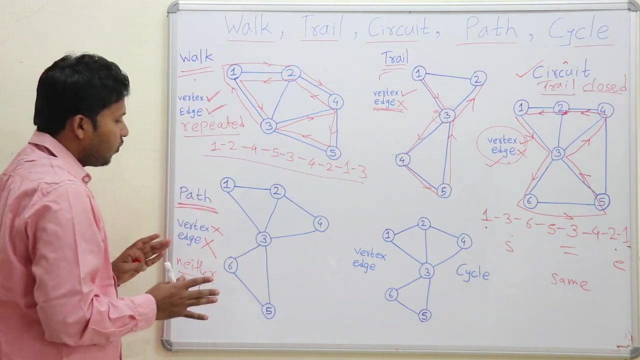 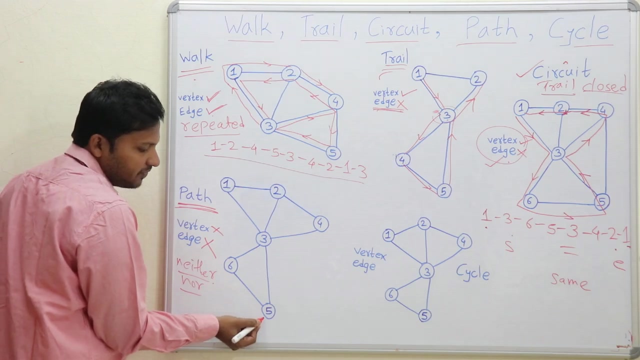 edges also cannot be repeated Means neither vertex nor edges. Neither vertex nor edges can be repeated. Okay, So vertex cannot be repeated and edges cannot be repeated. So let us perform a traversal here, which is a path. So let us start. So here you start from 5. See, the starting vertex can be any vertex to perform any traversal. 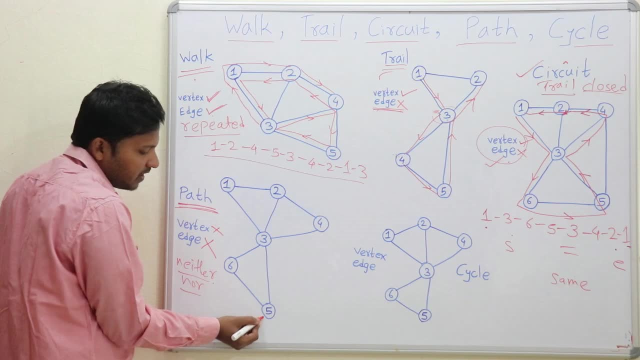 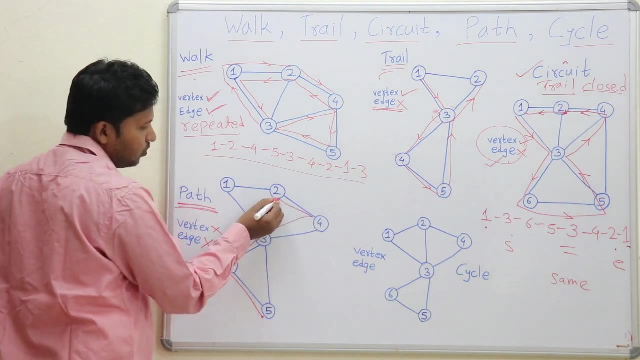 in a graph. Okay, So see: Start from vertex 5, from 5 to 6, then on 6 to 3,, then suppose, from 3 to 4, 4 to 2, 2 to 1.. Okay, From 1 to. 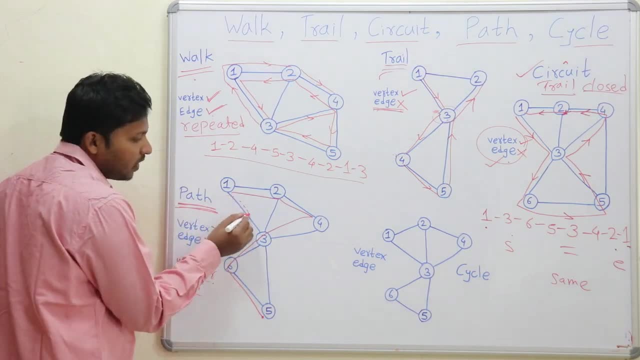 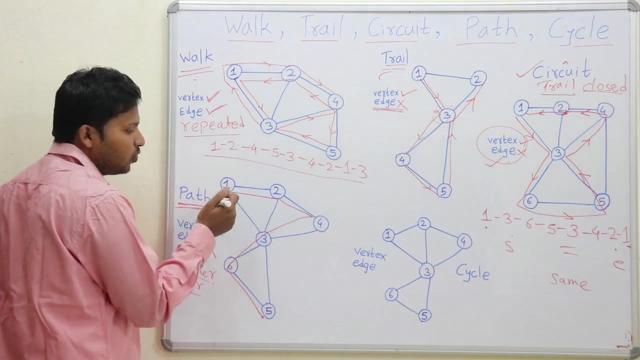 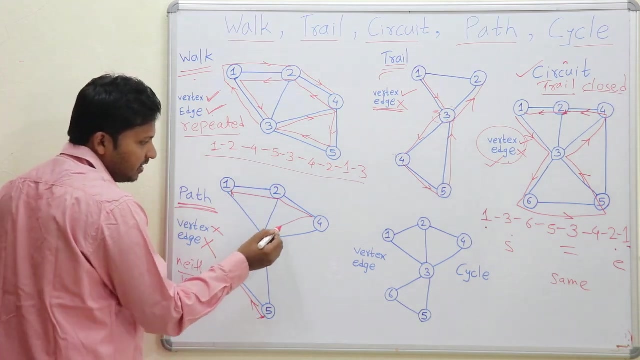 3,. you cannot go, because if you go from 1 to 3, that vertex 3 will be repeated. So you cannot go from 1 to 3.. So here you have to end the path. Okay, So the path is from 5 to 6,, from 6 to 3, and from 3 to 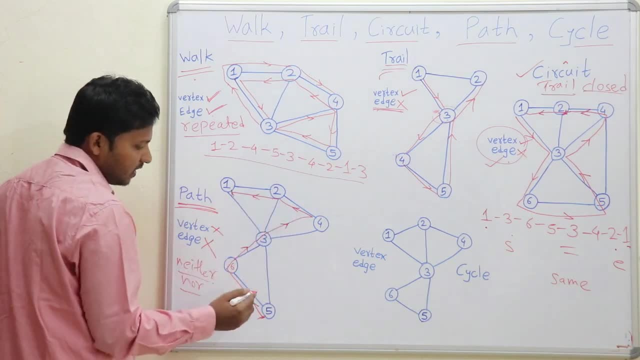 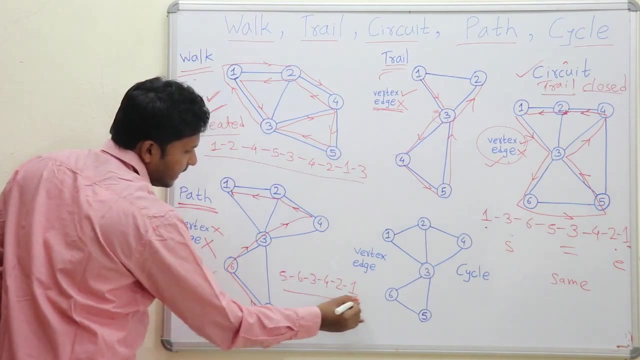 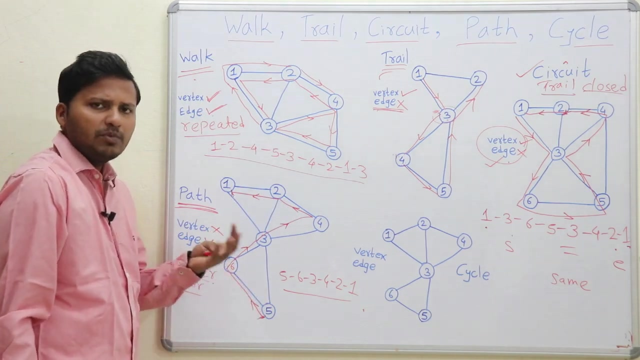 4, then 4 to 2 and 2 to 1.. So let us write C: 5, 6, 3,, 4, 2, 1.. So this is the path in this graph. There can be many paths in a graph. There can be multiple paths in a. 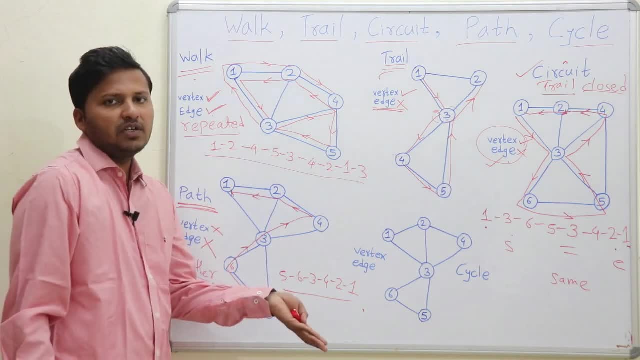 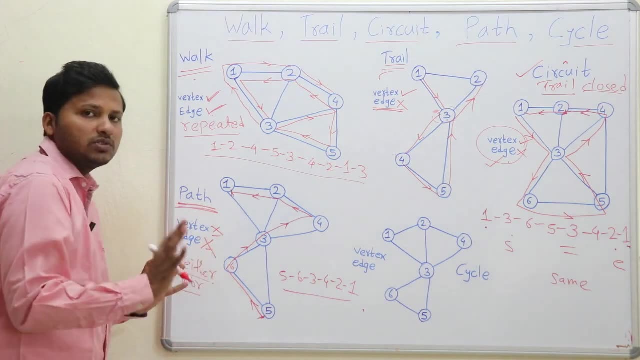 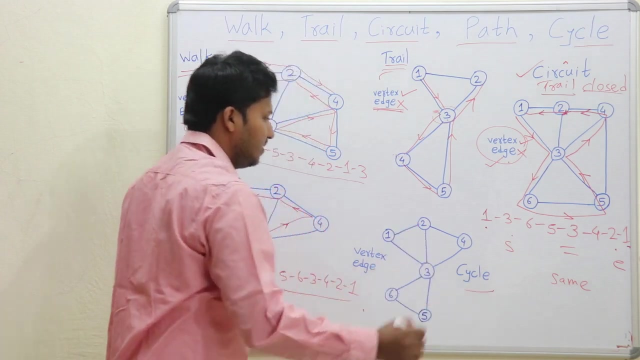 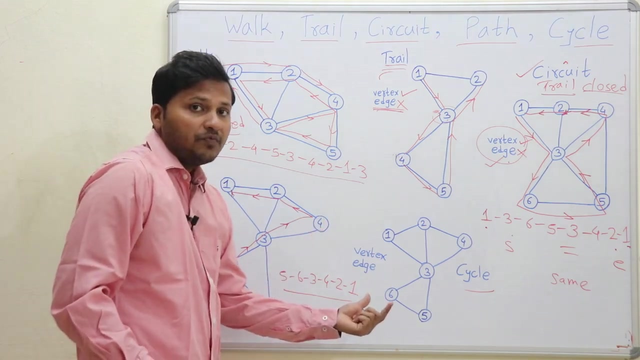 graph containing different number of edges and different number of vertices. So C in a path, vertices and edges. both cannot be repeated. Now let us go for a cycle. What is a cycle? So a cycle is a path, means it satisfies all conditions of a path with an